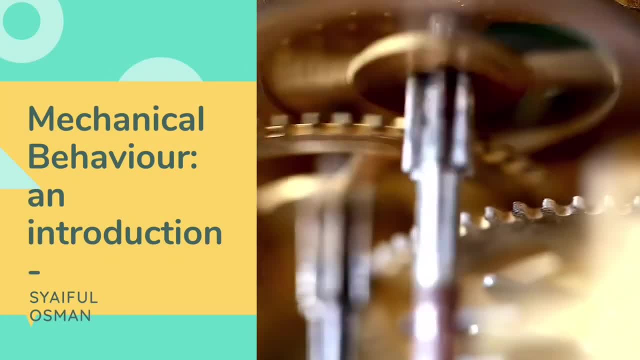 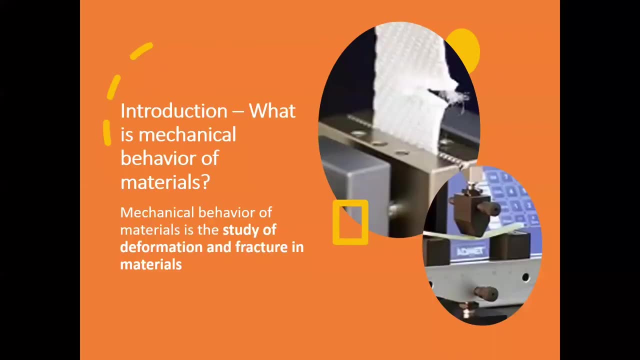 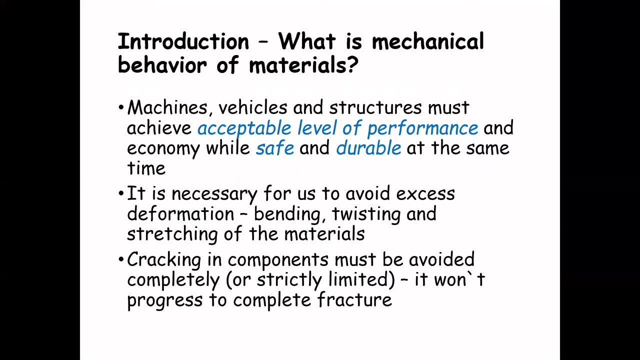 The study of deformation in fracture materials is called mechanical behaviour of materials. The knowledge of this area will provide the basis for avoiding these types of failure in engineering. application Machines, vehicles and structures must achieve acceptable level of performance and economy, while safe and durable. at the same time, It is necessary for us to avoid excess deformation. 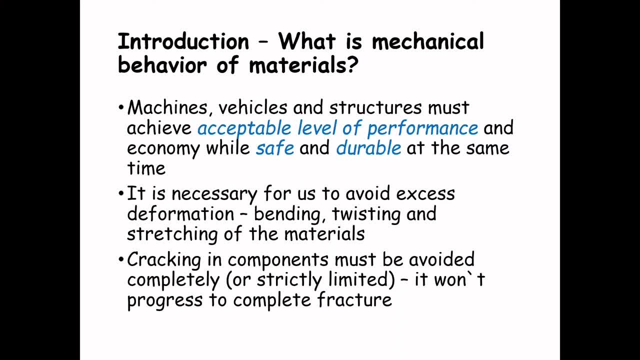 such as bending, twisting and stretching of the materials. Breaking in components must be avoided completely or strictly limited so it will not progress to complete fracture. Basically in mechanical behaviour of materials, topics that will be covered include elastic and plastic deformation create fracture and fatigue of materials, including crystalline. 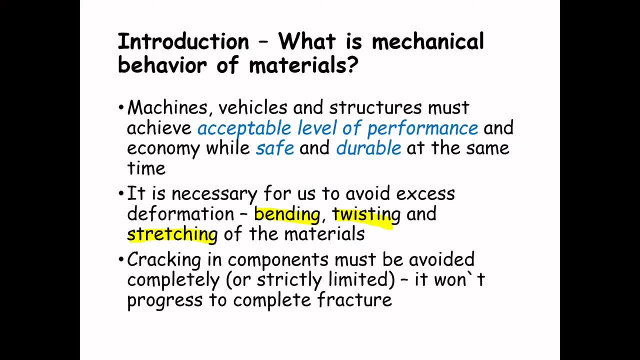 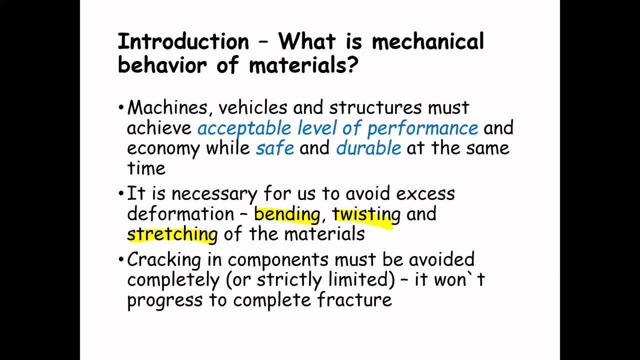 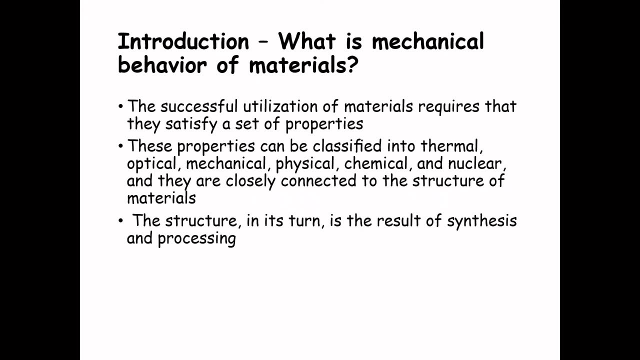 And it will focus on the design of the material, And it will focus on the design and processing of materials from the atomic to macroscale to achieve desired mechanical behaviour. So why do mechanical properties important? Material testing is often the last step in the manufacturing process, and yet the quality 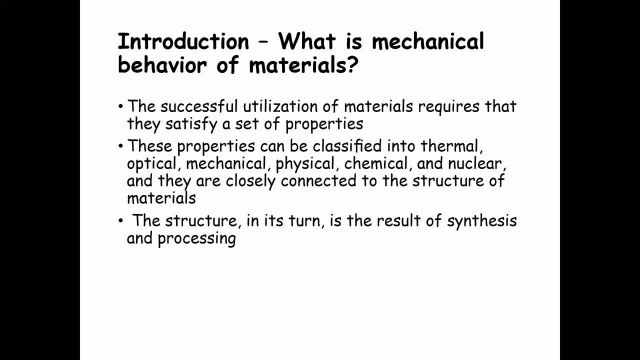 is the result of both the process, the process and the material. if the material that goes into the product is defective, then the product may be defective. so in the process of forming materials, understanding the materials properties can help to better predict the manufacturing outcome. and for our manufacturers it is very important to understand the mechanical properties of materials. 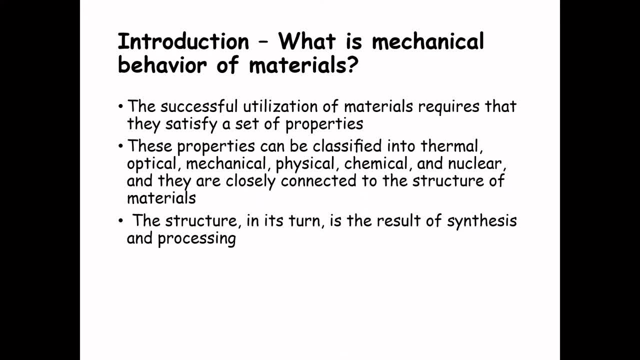 that exhibit some hookian behavior during loading. it is important because the performance of a structure is frequently determined by the amount of deformation permitted, and some measured properties that must be considered when we want to design something or when we designing a structure include a tensile strength, yield strength and young modulus of elasticity. 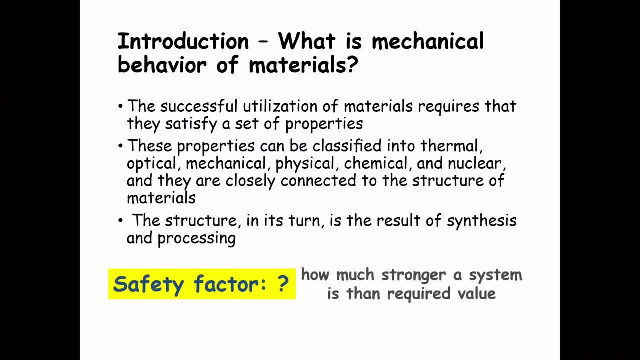 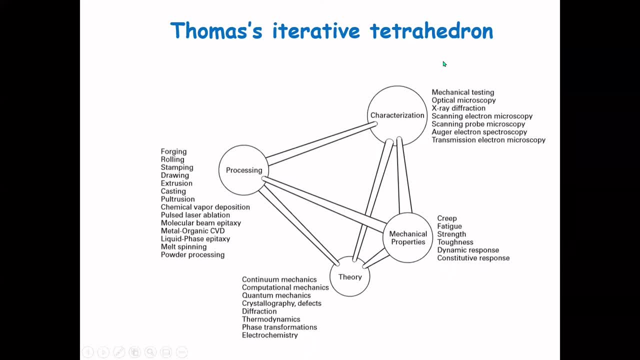 and the. the tetrahedron is a schematic framework that explain the complex relationship in the field of mechanical behavior or materials, the successful utilization or application of a material. in the field of mechanical behavior or materials, the successful utilization or application of a material material requires that they satisfy a set of property, and these properties can be classified. 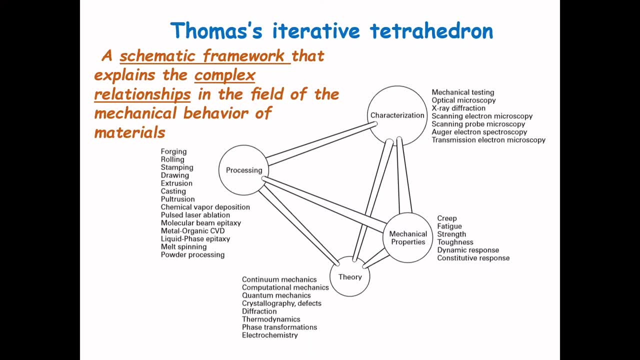 into thermal, optical, mechanical, physical and nuclear, and they are closely connected to the structure of materials, and the final structure is the result of a synthesized and processing. so a schematic framework that explains the complex relationship in the field of the mechanical behavior of materials is what we call as a thomas iterative tetrahedron, which contains four 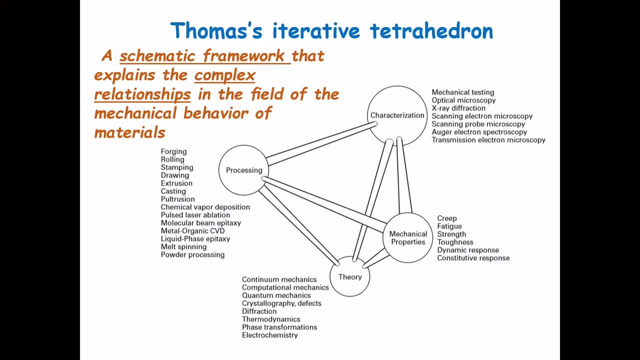 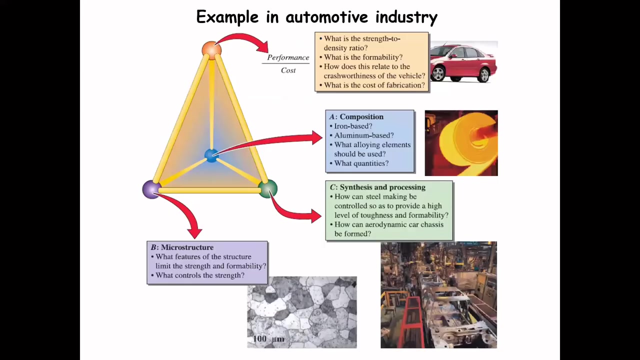 principal elements, that what we can see in the figure. here we have a mechanical properties, we have a characterization, we have a theory and we have a processing, and these elements are related and change in one will affect the changes in others, and so we have an example of thomas. 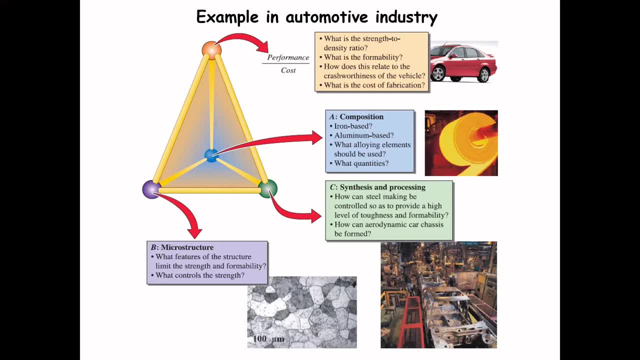 iterative tetrahedron in automotive industry. the application of the tetrahedron of material science and engineering to produce a sheet stills for automotive chasis. and we can see here, we note, that the composition, the microstructure and the synthesize and the processing are all 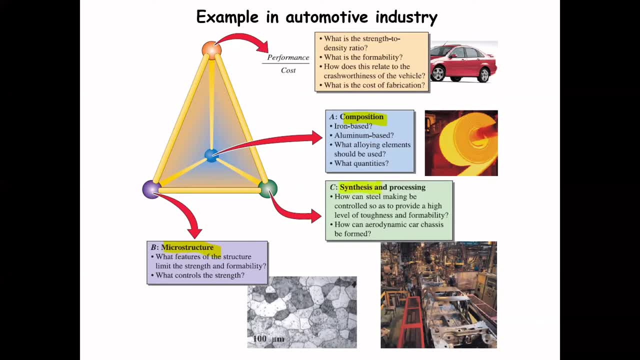 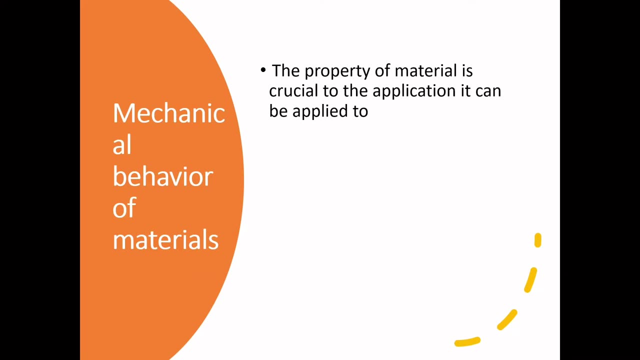 interconnected and in the end i will affect the performance to the cost ratio. the property of material is a crucial to the application but it can be applied to and it is very important and necessary for the design specification: deformation and failure estimation, microstructure, property relation, selection of the material and also in the design specification. 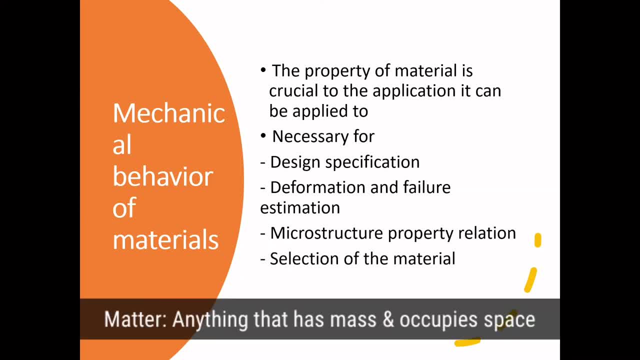 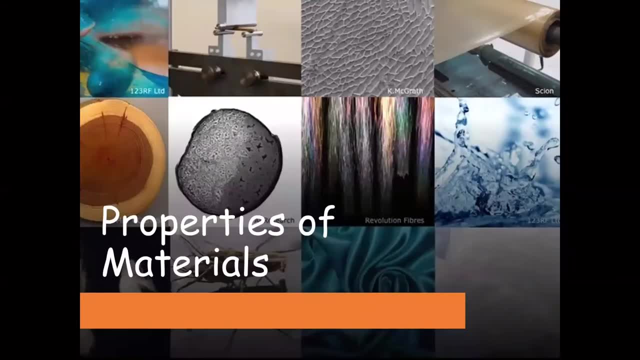 and also in the design specification and the failure estimation, microstructure property relation. in terms of economic consideration, matter is anything that has a mess and occupies a space, and a useful way to start thinking about a matter is to think about the different materials or substance that it can. 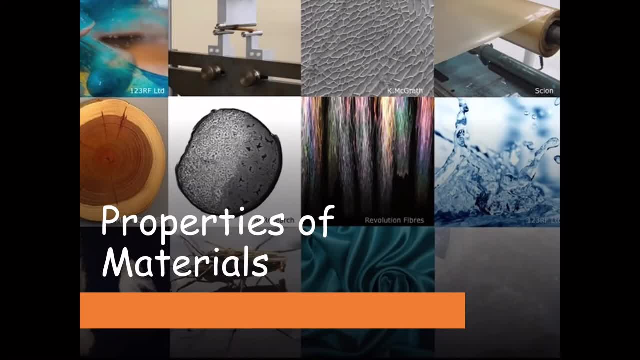 be made into and these materials make up the object about us, and each of these materials has a different properties or characteristic that can be observed or tested. scientists, technologies and engineers investigate these materials, they experiment with them and compare them, compare their properties and relate the result to a possible users. 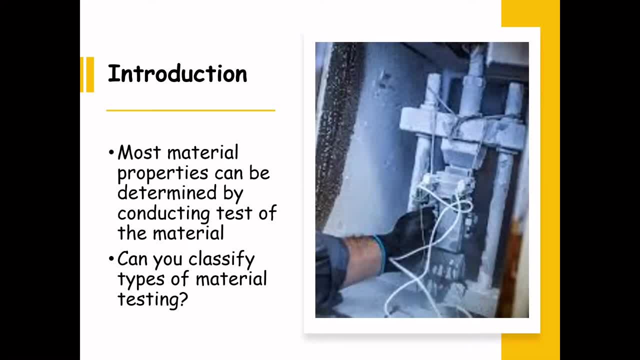 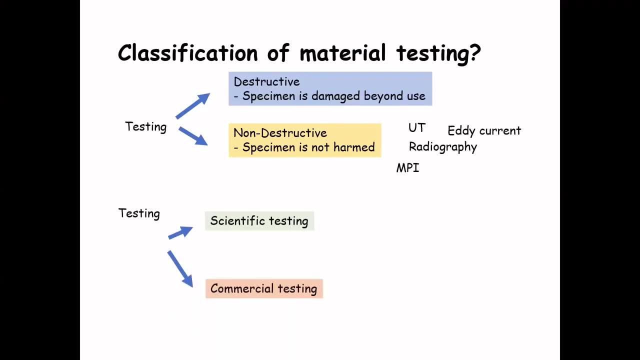 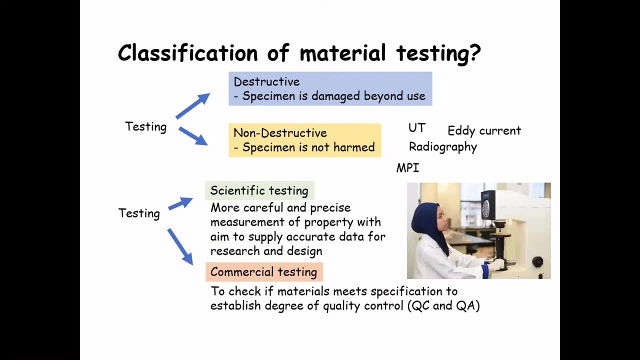 so now we will talk about testing of materials to determine its mechanical properties. so now we will talk about testing of materials to determine its mechanical properties. so here is how we can classify our material testing. first, we can classify materials testing based on destructive and non-destructive testing. so in destructive testing this specimen is damaged. 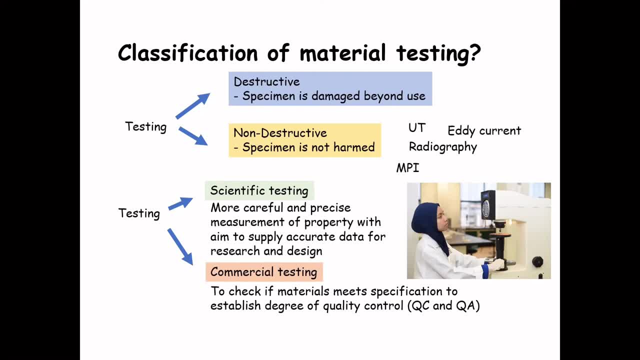 beyond use. for examples, we have a bending testing, tensile testing and impact testing. that are some examples of destructive testing. non-destructive testing, on the other hand, is where the material is not damaged or harmed. for examples, if you want to determine the structural integrity of pipeline, entity is the most suitable way for that purpose, and here we have some examples of. 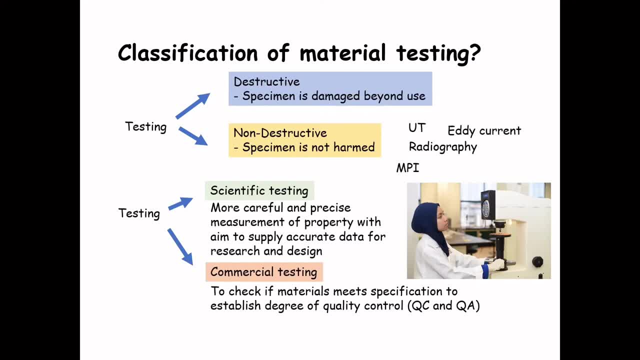 entity testing. we have ultrasonic testing, we have any current, we have radiographic testing, we have and we have magnetic particle testing and also we can classify testing of materials based on scientific testing and commercial testing. in scientific testing, more careful and precise measurement of a property with aim to supply accurate data for research and design, and on the other hand, we have a 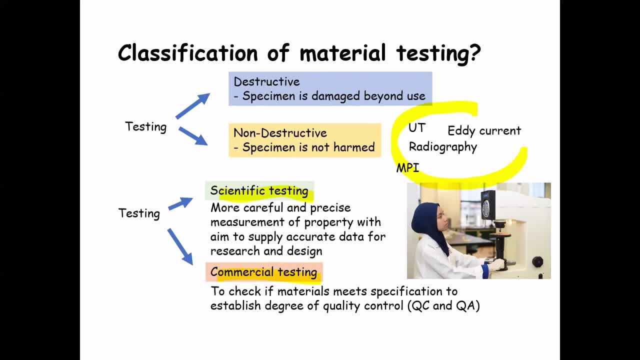 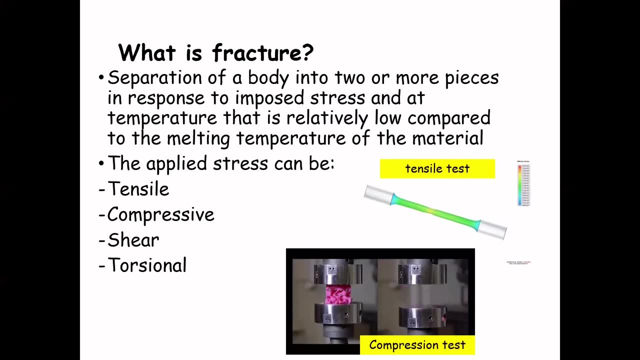 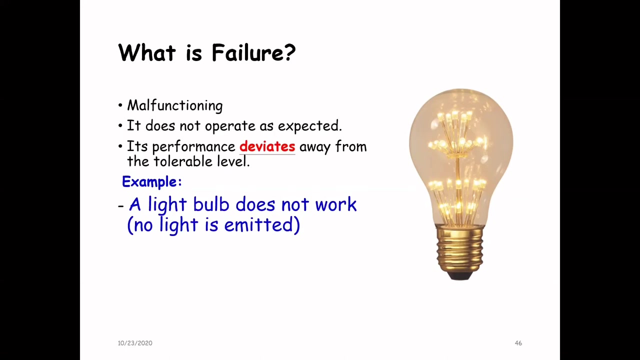 commercial testing with the purpose to check if the materials meet this specification to establish a degree of quality control. we don't want engineering materials to fail because they can cause loss of life, economic loss or a loss of a product or services. The usual causes of material: 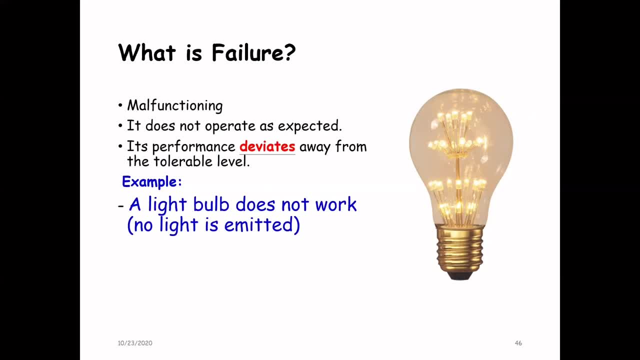 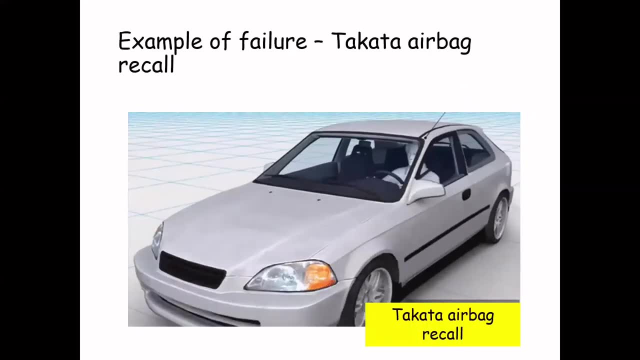 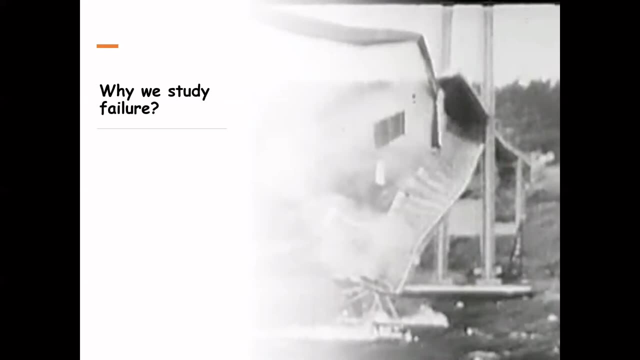 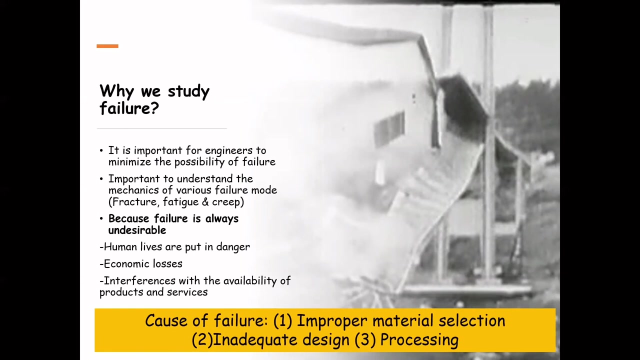 failure are incorrect material selection, incorrect processing, incorrect manufacturing procedure or inadequate design. Failure is defined as any change in size, shape or material properties of a structure, a machine or machine parts, or in other words, a part become unable to satisfactorily perform its intended function. It is important. 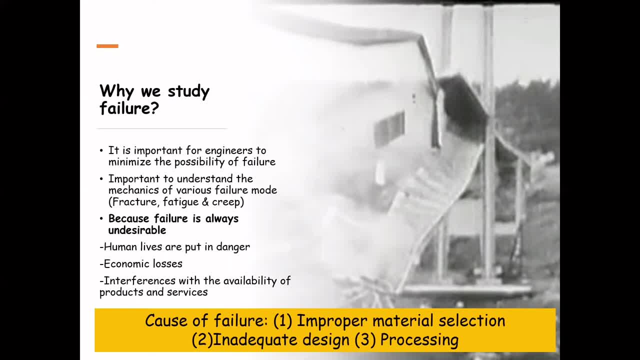 to understand the mechanics of various failure modes. Failure is always undesirable because it will put human lives in danger, it will cause economic losses and will interfere with the availability of a product and services. And commonly the causes of failure are improper material selection, inadequate design and also processing. 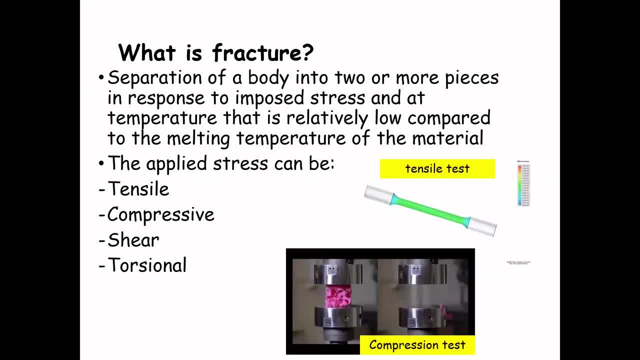 So first, maybe it is important for us to define what is a fracture. We can define a fracture as a separation of a body into two or more pieces in response to applied stress at a temperature that is relatively low to the melting temperature of the material. So how does a fracture occur? 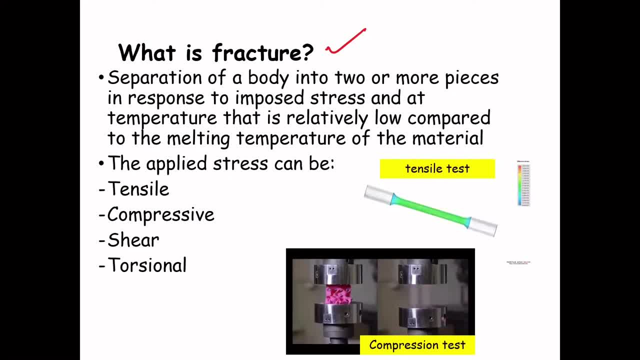 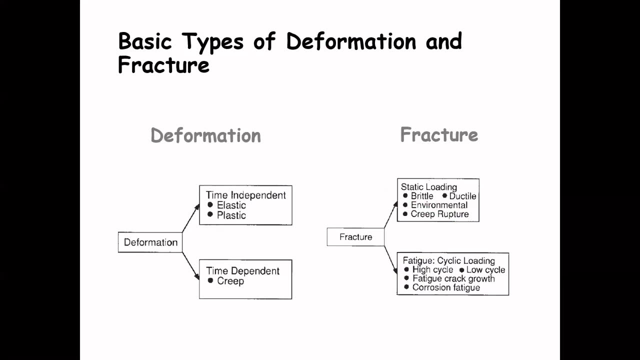 Fracture occurs when the metal or material experiences a stress that exceeds its yield strength. Fractures can occur in three different types, that is, a ductile fracture, moderately ductile fracture and a brittle fracture. So deformation can be divided into two, that is, a time-independent, such as elastic and plastic, and also a time-dependent, such as a crib. 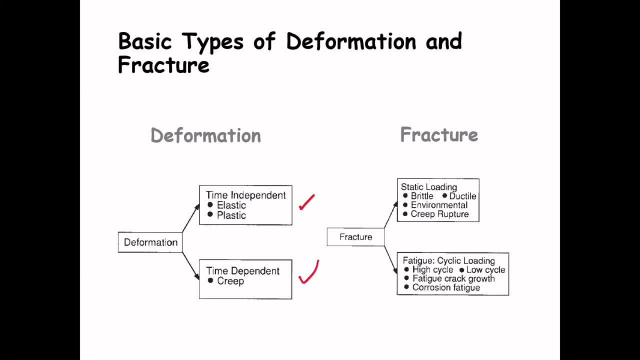 Fracture, on the other hand, can be due to the static loading that is, either brittle or ductile, due to environmental and the crib rupture. And in addition to that, fracture can also be due to the fatigue or cyclic loading that is either high or low cycle and crack growth can occur during fatigue. 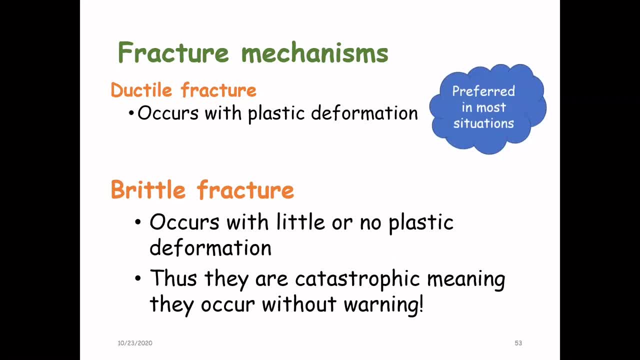 So now I want to talk about a ductile and a brittle fracture. So we have a ductile fracture that can be defined as a fracture that occurs without plastic deformation, And this is the most preferred in most situations. And then we have a brittle fracture that happens with little or no plastic deformation. 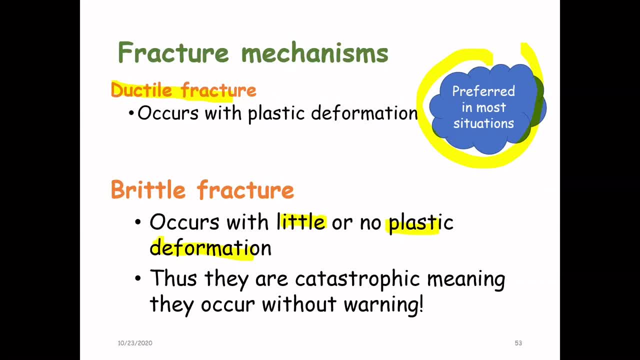 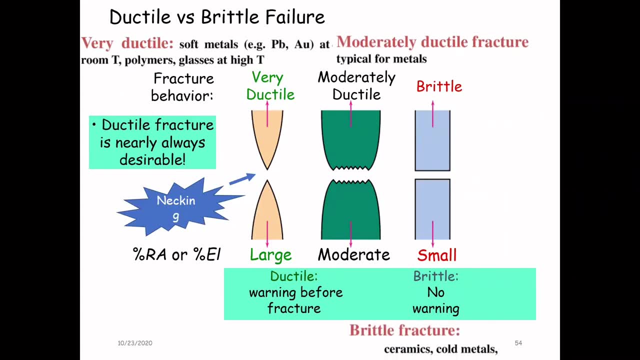 And thus they are catastrophic. They can occur without a warning, And this is how we can show a fracture behavior of a very ductile, moderately ductile and a brittle material. And so we can see here, for a very ductile material, the specimen neck down to a point here in the middle. 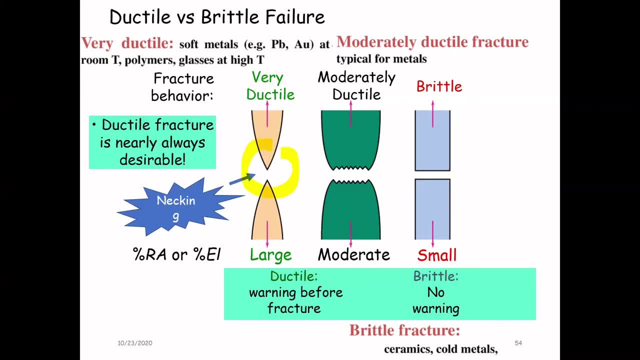 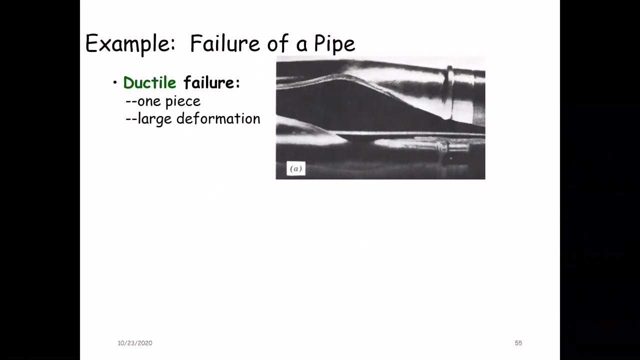 And here we have a failure for a moderately ductile material. And then we have a very we have a brittle material here where we can see that deformation is very small And a fracture occurs without a warning. And here we have an example of a failure of a pipe.